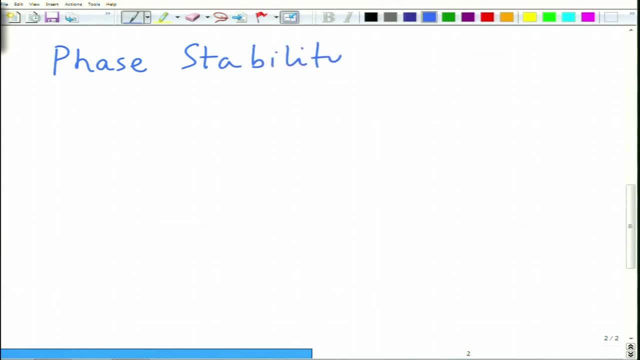 Stability, Phase stability, basically, is determined by thermodynamics And in particular, so basically what we are looking at at a given condition of given temperature. So what are the pressure and composition, What are the stable phases And this is what is phase equilibria. 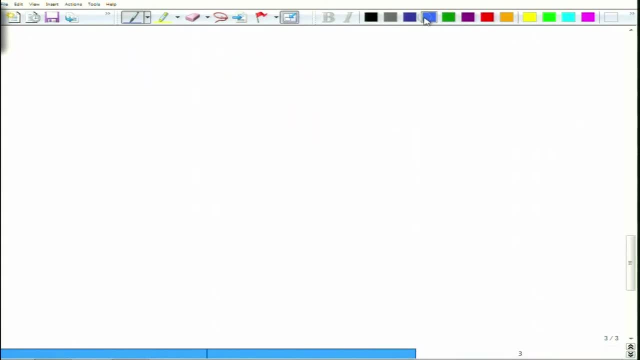 So let us first define the term called as free energy. So I assume that you have basic knowledge of elementary thermodynamics, Elementary thermodynamics, which is useful to understand the course. So free energy, so at a constant, at a given temperature and pressure, as well as composition, Free energy. 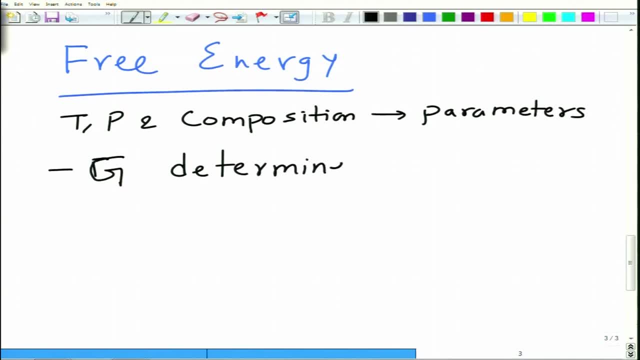 G. this is G determines. G determines is the phase stability for an alloy and G is called as Gibbs free energy, and this G is written as. G is written as H minus T, S, So H is called as enthalpy, T is the temperature. 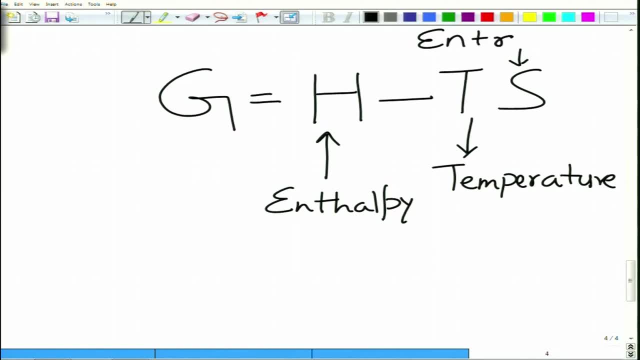 and S is called as entropy. So now just let us just look at the definitions of these components. So let us first look at what is enthalpy. So enthalpy is essentially defined as H. it is essentially defined as: 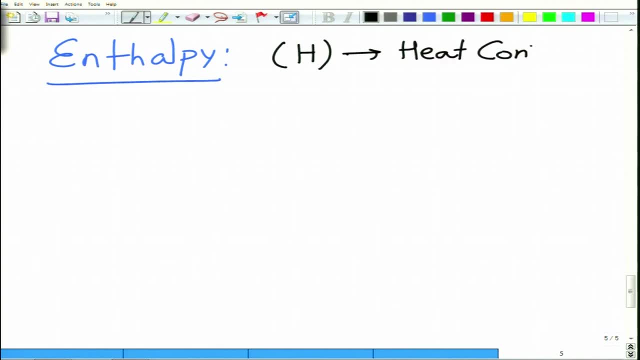 heat content of a given system. So this is the energy inbuilt in a system which consists of the internal energy and which consists of the pressure and volume terms, the net amount of work which is done by the system or on the system and that will determine the total heat content of the system. 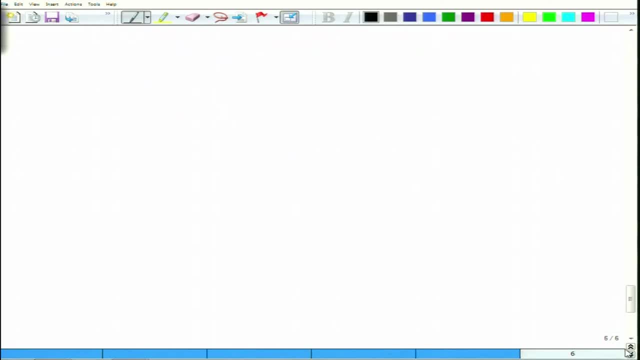 So let us now first look at the internal energy. So this U is basically sum of all the kinetic energy contributions and all the potential energy contributions. So this U is basically So kinetic energy may arise from, let us say, A- atomic vibrations, B. it could be due to: 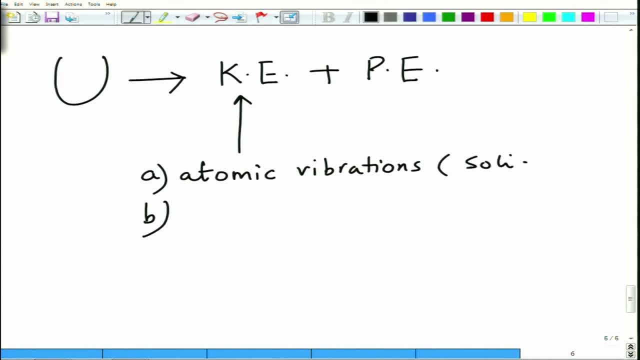 so atomic vibrations in both solid and liquid phase. It could be because of translational, So it is very valuable, and rotational energies of atoms or molecules, So it again could be within the liquid phase or gas phase. generally these are more of significant liquid and gas phase, whereas atomic vibrations. 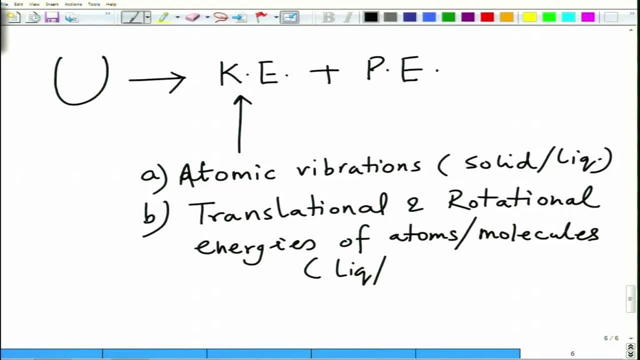 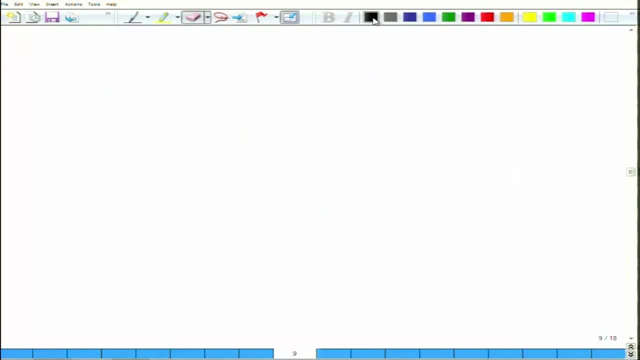 are more in gaseous phase. So this is the kinetic energy term. The potential energy term, on the other hand, is written as follows: So this is potential energy term, is potential energy Pe, which is because of, which is due to bonding, It is also because of atomic or 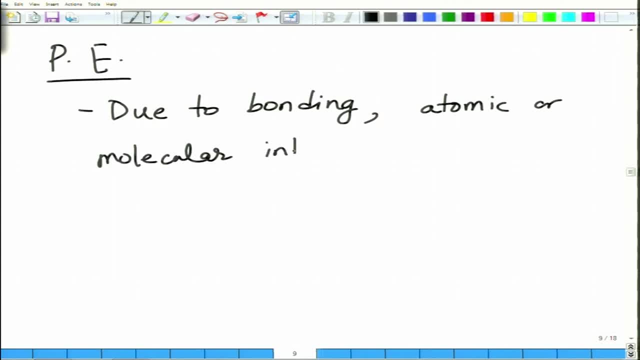 nuclear interactions, because it may not be only bonding, it could be various other things such as hybridization and things like that interaction in a system. So this is what the total energy now will be. So you have kinetic energy and then you have potential. 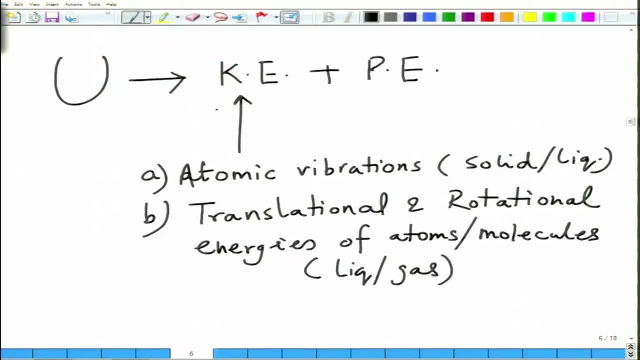 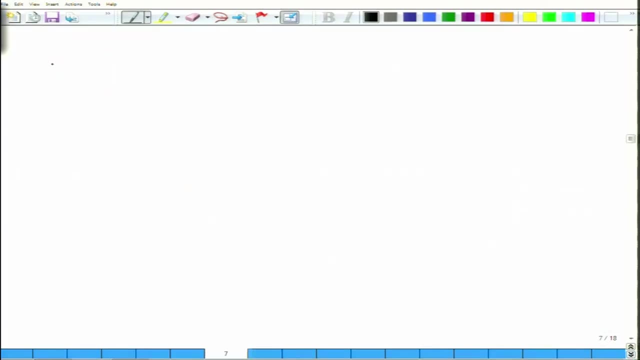 energy. Now let us look at the total energy is equal to kinetic energy plus potential energy. The kinetic energy is because of atomic vibrations and so which are basically which in solid and liquid, both forms, as well as translational and rotational energies of atoms and molecules, whereas potential energy is because of, as I wrote just now, is because 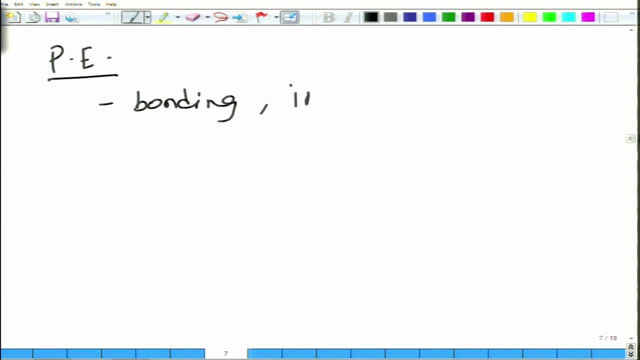 of bonding and inter atomic interactions. So this gives rise to total energy. So total energy now would be Ke plus Pe. So basically, as you change the temperature, the internal energy increases. Now why does it happen like that? So when you go from, for example, water to vapor, for instance water, 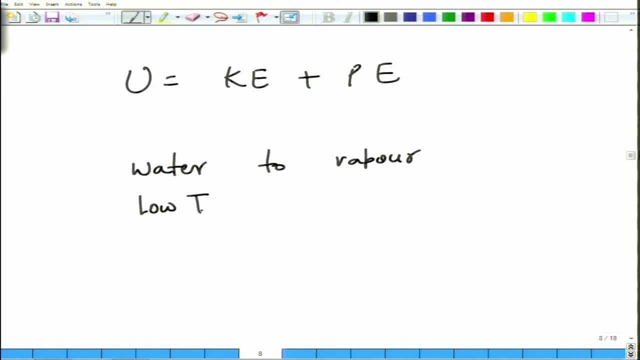 to vapor. essentially you go from low temperature to high temperature and basically you are adding heat to the system. So your internal energy will go up, and then you will say that you will stop your energy formation. So this will stop your energy formation. So this is the internal energy. so, basically, 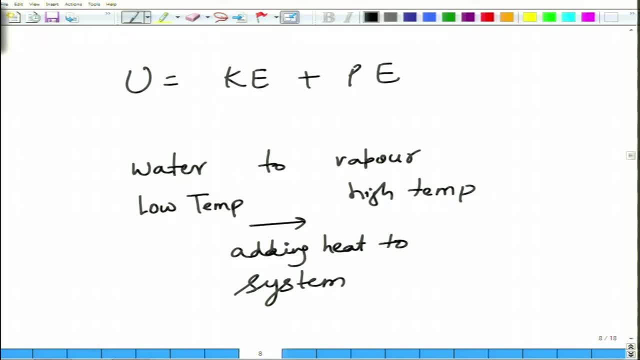 you go from vapor to vapor, The internal energy will go up, and then your internal energy will as you go from water to vapour. Similarly, let us say: if you heat a solid, you increase its energy because you add heat. Similarly, if you heat, for example, let us say tungsten. 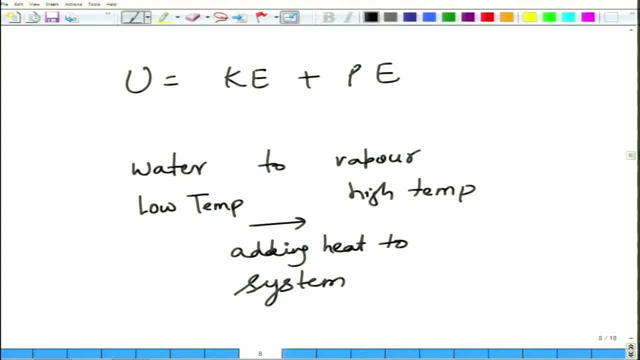 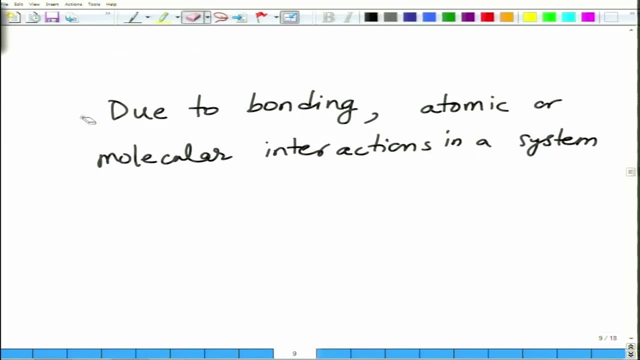 filament bulb, the tungsten filament becomes red hot and which means its internal energy increases and as it cools down, its internal energy decreases. So now, if I just give you the science of these energies, so if you have, let us say, a system, and then you have surroundings, and so, basically, if you do so, this is let us. 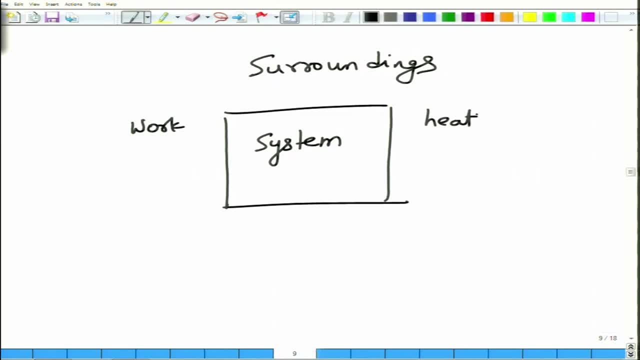 say: on this side you write work, on this side you write heat. So if work is done onto the system, then delta E is delta U. let us say delta U is positive. And if you do work on work, if system does the work, then delta E is negative. On the other hand, in terms 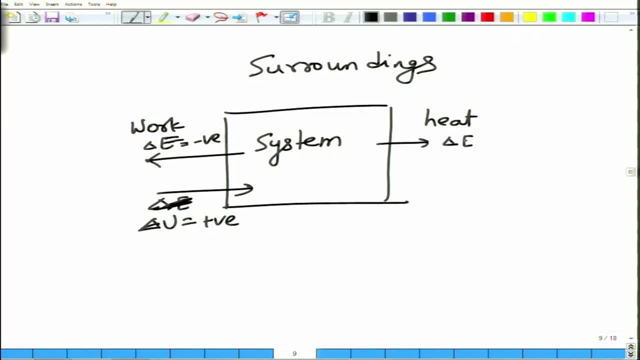 of heat. if system releases the heat, then delta E is negative, and if system absorbs the heat, then delta E is positive. So that is how you distinguish between various states of the system as you decrease or increase the temperature. Now second thing that we talk about is the P-V term. The P-V term is of importance because 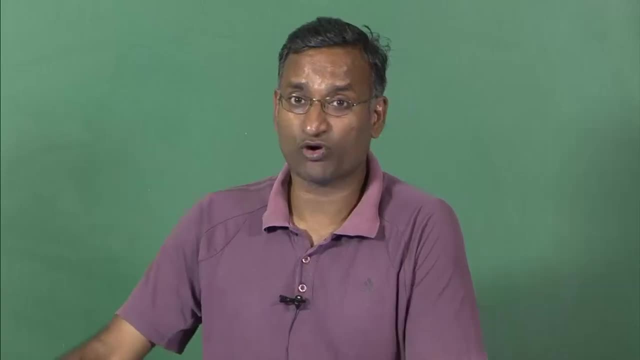 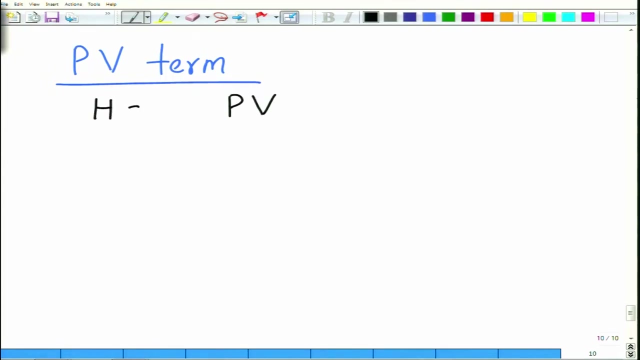 phase changes are affected by the change in the volume or the pressure. So when we say H, so this P, when we say H, is equal to U plus P, V. So it is this term which is the term which adds or which becomes plus or minus as come, depending upon the, what the 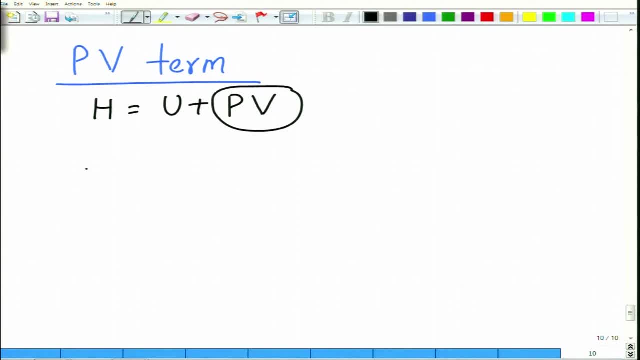 magnitude of this term is. So, basically, for mostly condensed phases in general, for condensed phases, condensed phases- by this I mean generally liquids and solids, The, The, The, the delta, P-V term is generally very small and hence it is generally neglected. So for 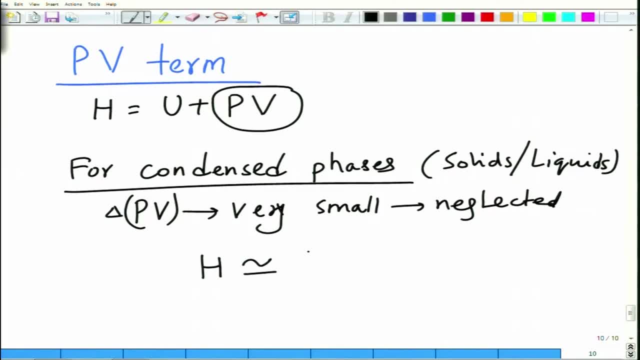 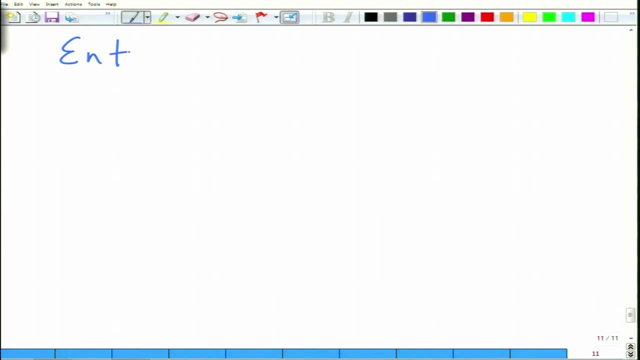 condensed phases. generally, H is nearly equal to you can say U if this delta P-V term is very small. And finally we come to the third term in G minus TS, that is, that is what is called as entropy. this entropy is nothing. 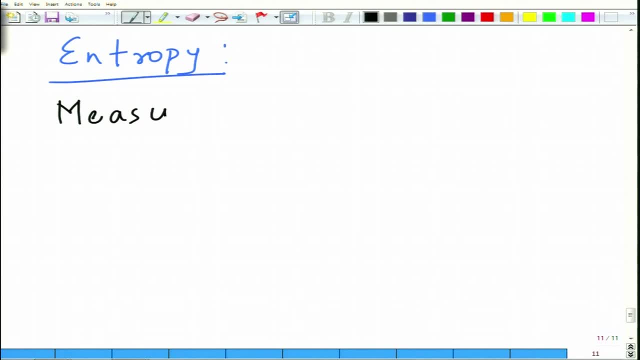 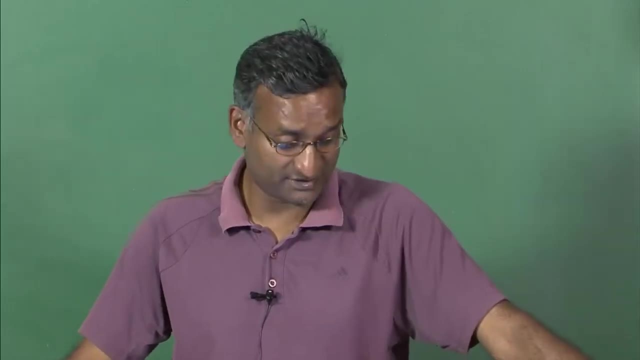 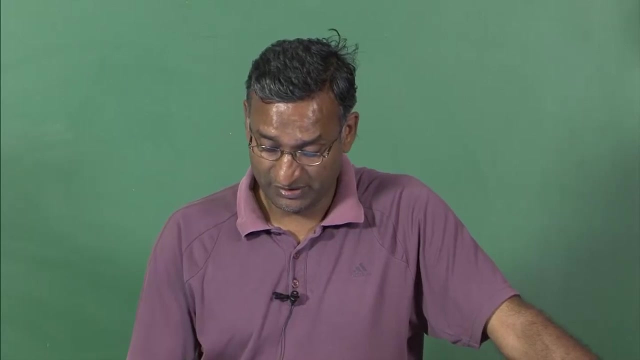 but a measure of randomness, measure of randomness or measure of disorder of species within a given system. and a- this is this- again- has a strong bearing on the overall stability of the system. So, but what we are doing, This the system. So as now we come to the first expression again: G is equal to H minus T s. 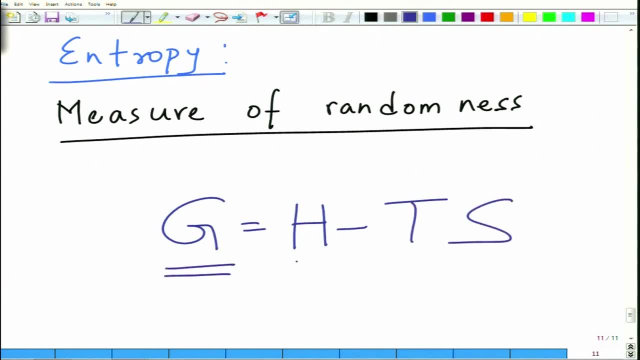 the free energy of a given phase is affected by the overall heat content, H, which is equal to U plus P, V. In most cases it is equal to U for solid phases and then T s term. So whether enthalpy increases or decreases, or the entropy term increases or decreases under 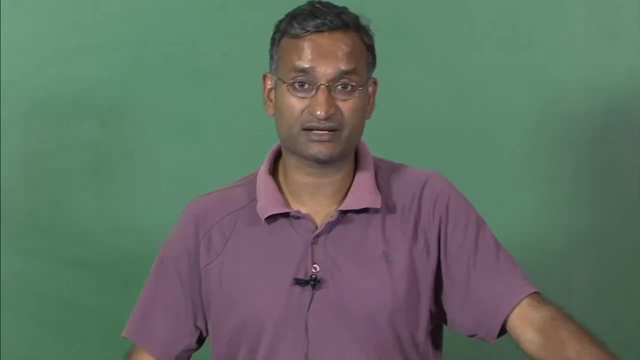 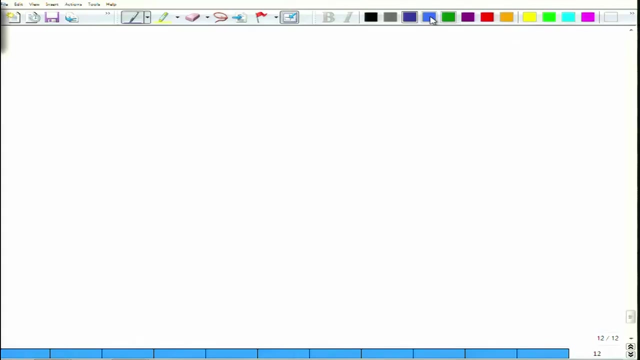 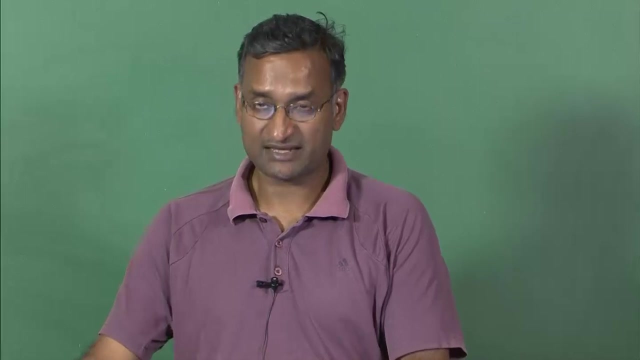 given set of thermodynamic conditions will determine whether G will increase or decrease as a function of temperature or pressure for a given system. Now let us look at the definition of what we call as equilibrium. So what is equilibrium? Equilibrium is defined by: generally, we defined as equilibrium as in the context of materials. 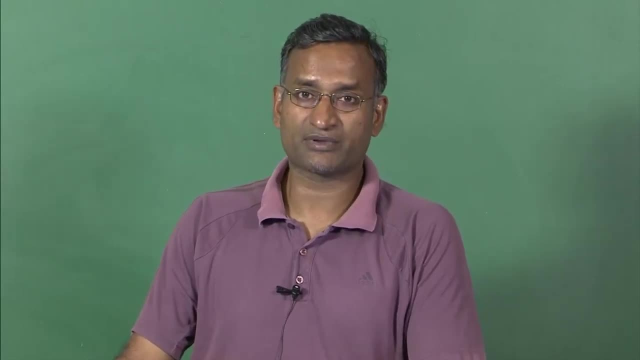 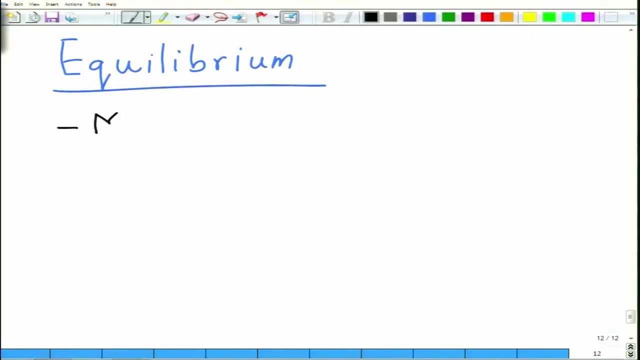 the most stable state. that is. no change happens if you leave the system on its own under given set of parameters. So basically, the you can defined equilibrium as most stable state of a system under given set of temperature, pressure and temperature. So basically, if T and P- you can define these- are constant, then dG is equal to 0. and what? 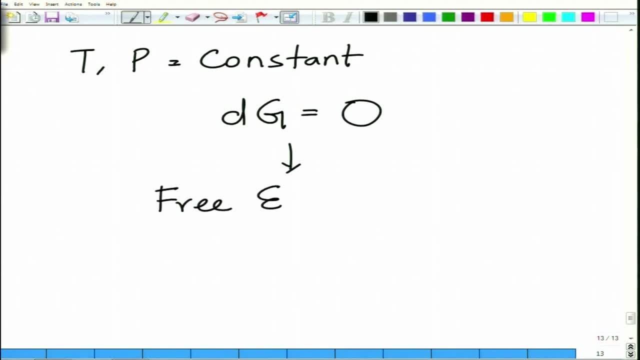 it means is that free energy has a minimum under those conditions. So generally, if you look at again, G is equal to H minus T s. so G will decrease when H is small. So if you decrease H, your G will decrease and when you increase entropy, G will decrease. 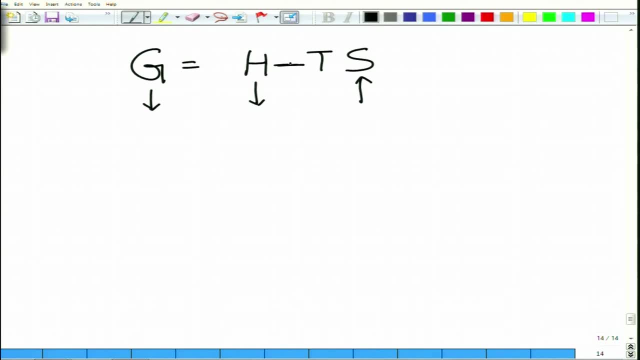 because there is a negative term. So, generally speaking, the free energy decreases when enthalpy decreases or entropy increases because minus T s term goes as negative and H term. of course it has to decrease for the, but overall it is a combination of these two which will govern whether free energy will. 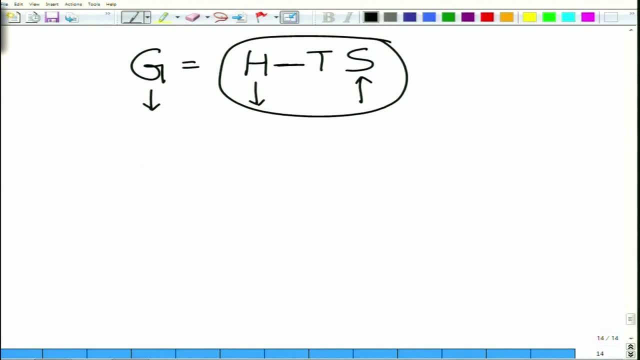 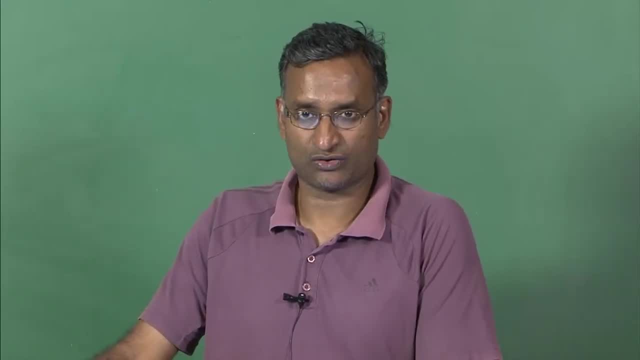 increase or decrease for a given system and generally, what we are interested in knowing: what is the relative change in free energy for given phases? So it might happen that you have two phases and, as the function of temperature, the free energy of both phases decreases. But if the decrease in the free energy for one phase is happening at a higher rate as compared to the other phase, then we may come across a temperature at which the free energy of the phase for which the energy decrease rate was higher may lead to lower free energy. 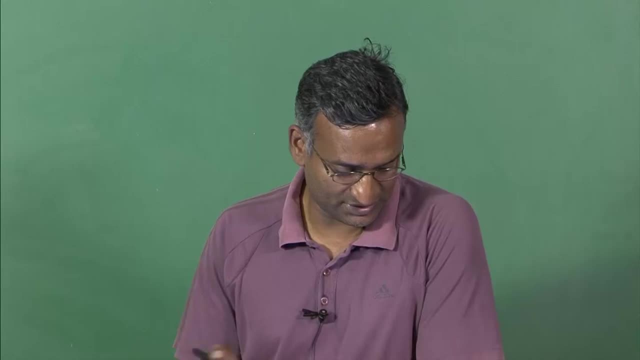 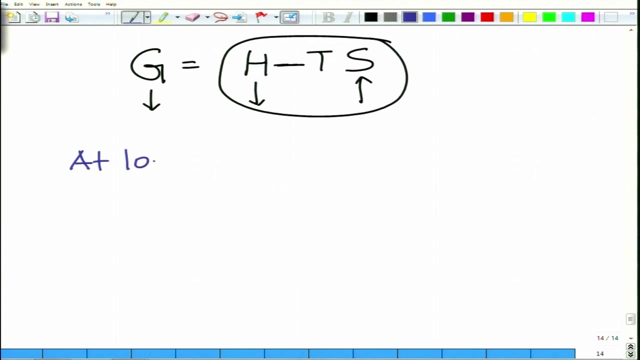 as compared to the other phase phase. So we will see those changes later on. So generally, so let us say, at lower temperatures, generally, what happens is that at lower temperatures, basically at lower temperatures, you have higher atomic interactions, and higher atomic interactions will lead to higher binding, stronger binding, and this 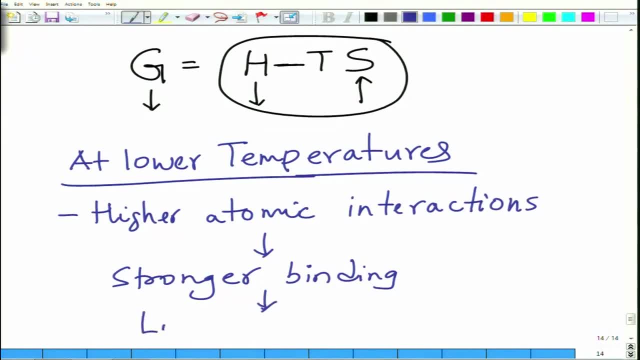 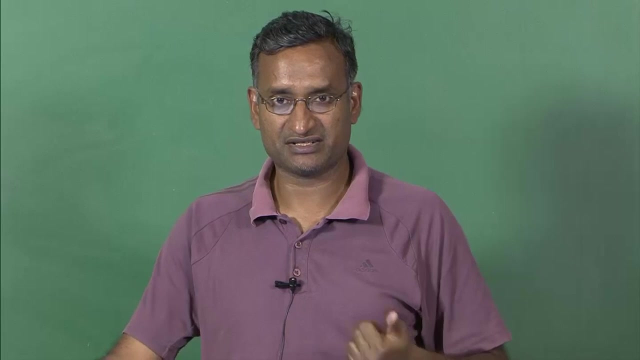 generally leads to lower atomic interactions, Low or more negative, you can say, internal energy, because- and that is why solids have lower internal energy or more negative internal energy as compared to the liquid gases have. if you compare solid liquid and gases, solid will have the most negative internal energy. 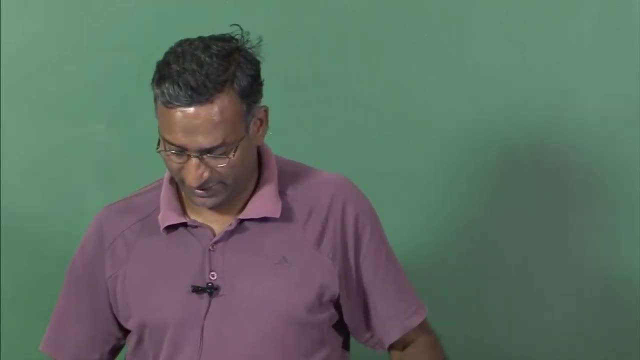 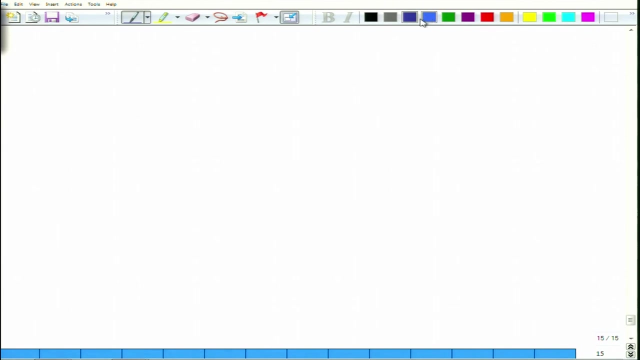 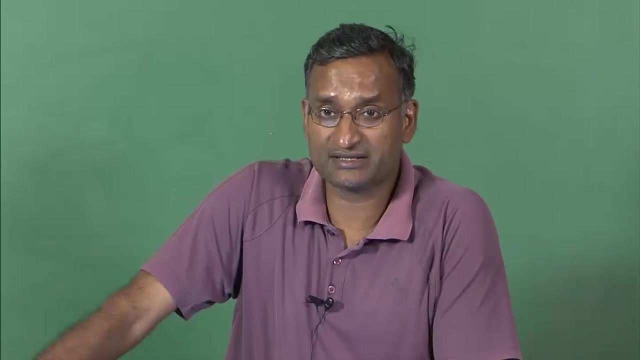 whereas solids and gases will have higher, more positive internal energy as compared to the solid. So, as a result, generally because of this decrease in the internal energy or negative internal energy of the solids, solid phases are more stable at lower temperatures. So 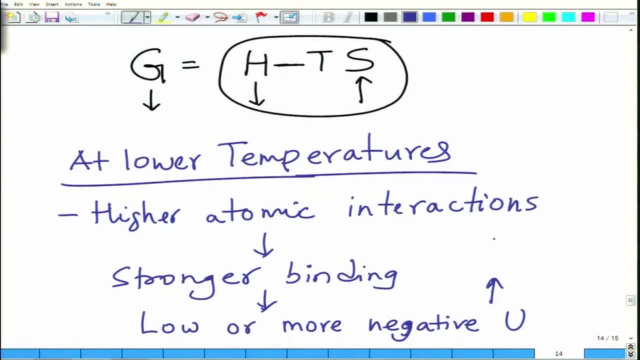 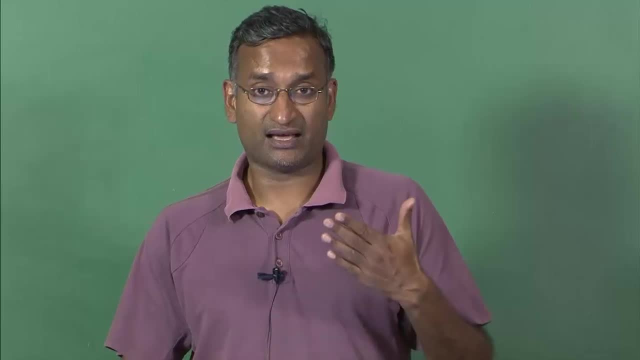 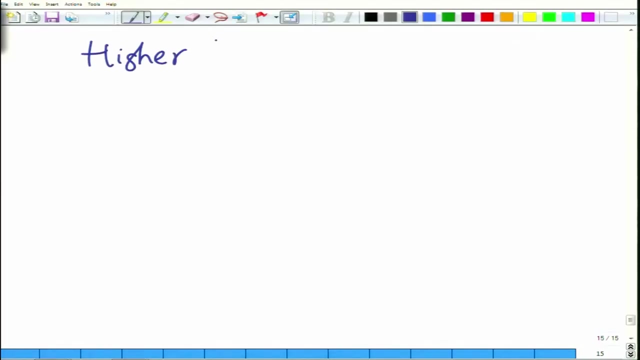 we can say, if you go to, this is what makes solids stable, whereas at higher temperature, conversely, at lower temperatures, solid phases are more stable at lower temperatures. So this happens: at higher temperatures your solids have your liquid and gases have although they have. So if you look at higher temperatures- higher temperature- we see generally liquids. 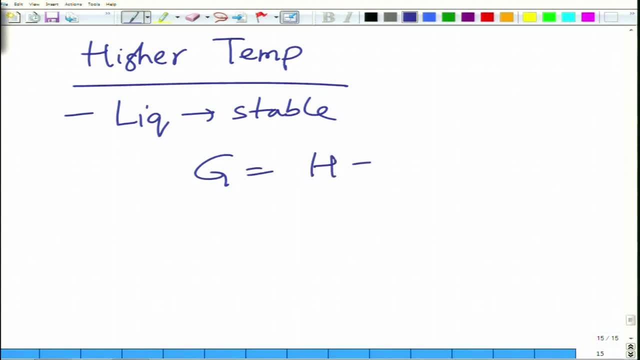 are stable, right, this happens- is equal to H minus T s, although their H is positive, although there is more, although the H is more positive as compared to the solids. solid, the entropy is higher. So, again, this entropy term dominates. this term dominates. 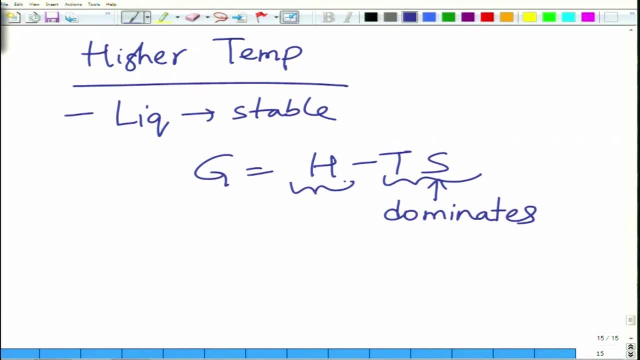 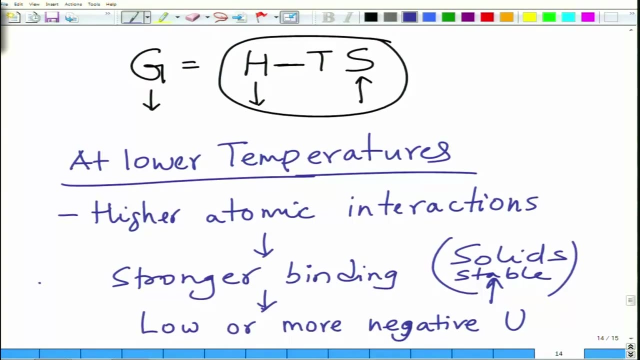 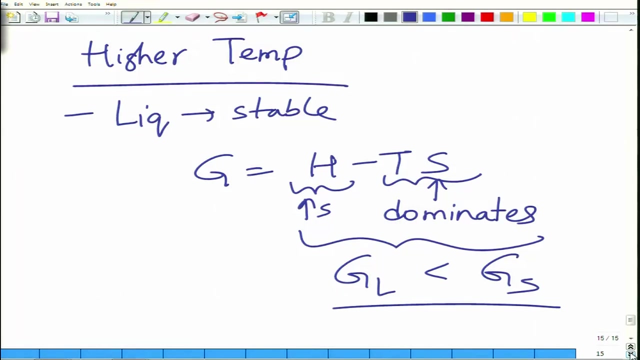 over the H term. So H increases but S also increases. So the competition between these two makes lower than G S, whereas at temperatures G S is lower than G L in general. So we will look at various systems, a few systems, later on. So at higher temperate term dominates lower. 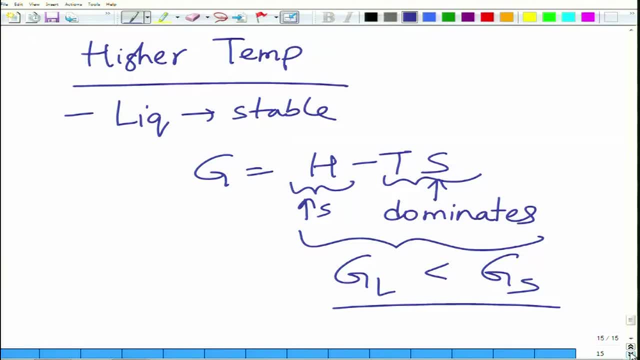 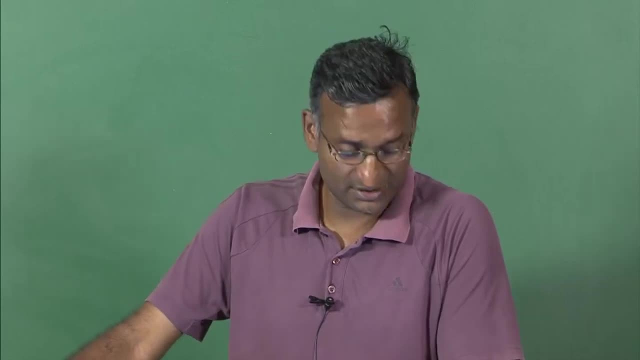 temperature, the enthalpy term dominates, giving rise to stability of solids and liquids at lower and higher temperatures. Similarly, you have pressure volume effect as well. As we said, generally, pressure volume effects are not generally considered but, however, if they are present, they have to be considered And hence the systems with smaller volumes are. 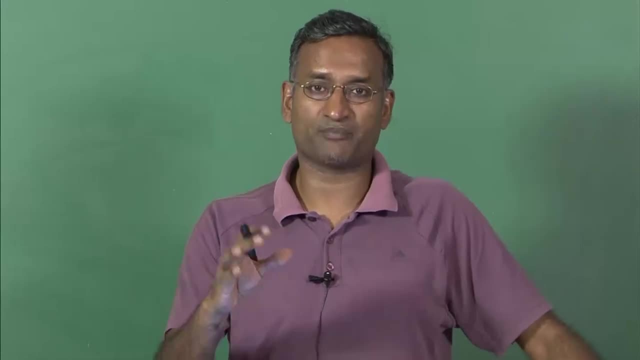 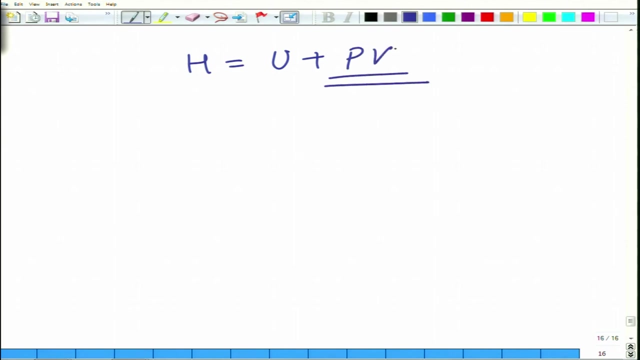 preferred as compared to the systems with smaller volumes. So these are the two systems as compared to system with higher volumes because of lowering of PV terms. So if you look at this, H H is U plus PV, So this volume term comes into picture at 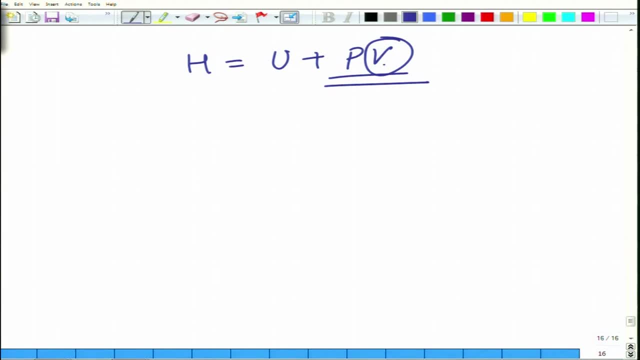 a given pressure. If you have two phases, the phase with a smaller volume will be preferred as compared to phase with higher volume, And this is because of changes in the corresponding changes in the enthalpy. So if your enthalpy has to at higher. so if you have two phases, another phase with 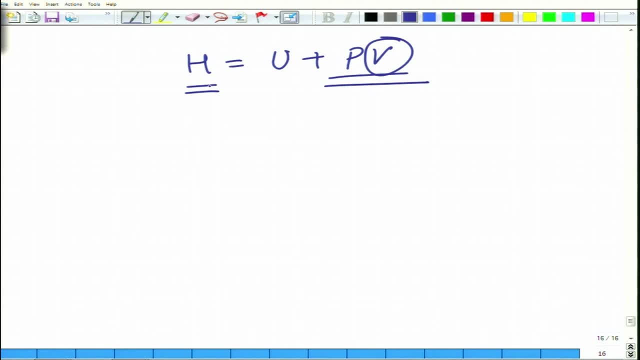 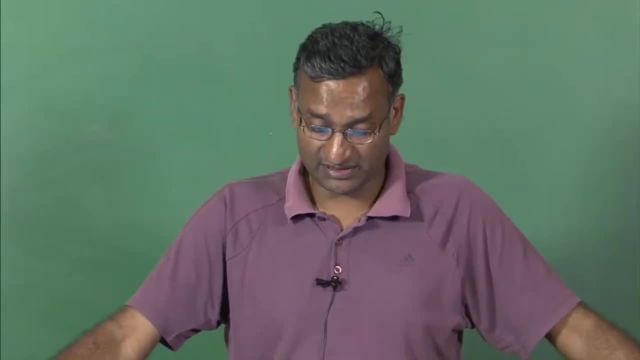 lower volume, that will have lower enthalpy as compared to the phase with the higher volume. So more negative enthalpy has to be will be preferred, or lower enthalpy will be preferred as compared to the, as compared to the other phase. 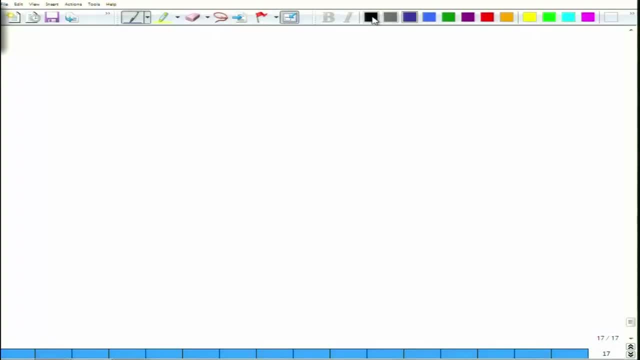 So when we define equilibrium in totality, the equilibrium in totality is defined as you have you plot G as a function of, let us say, arrangement of atoms. So if I make a plot of this, So this is for example the situation: you have a state A and you have 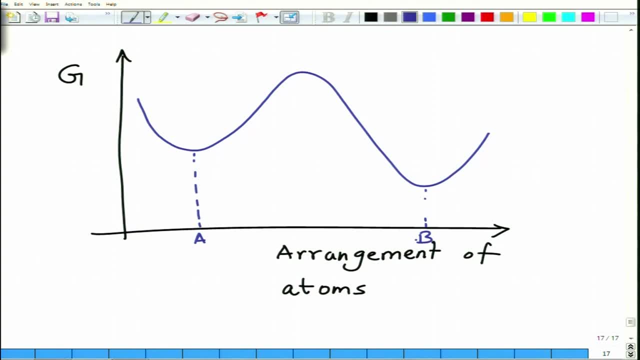 a state B. So you can see that there are two minima here. So dG for this is also 0, dG for this is also 0.. However, in totality, if you look at that free energy landscape, this B state has lower energy as compared to. So this is, let us say, Gb and this is. 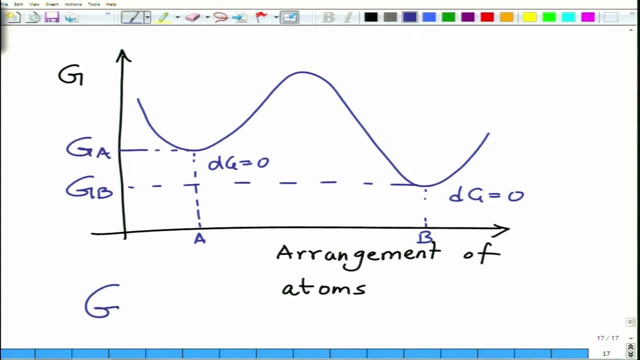 let us say Ga. So Gb is more stable at equilibrium because Gb is lower than Ga. So if you leave the state B, you can see that this B state has lower energy as compared to. So this system for long time to achieve equilibrium system will move towards achieving Gb. However, 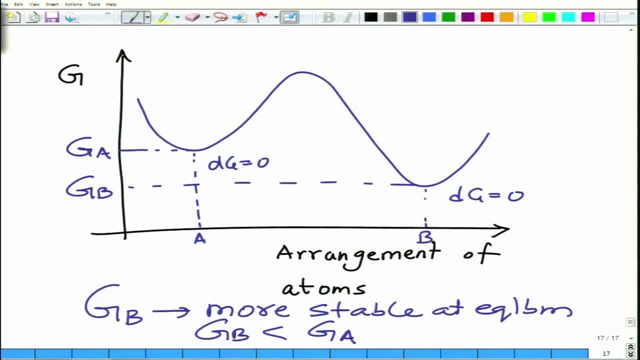 in many systems, such as in glasses, there are, or in polymers there are, metastable states which have local minima. So this local minima is often stable because this is also at an energy which is small. at this arrangement, However, to reach from here to here, it has. 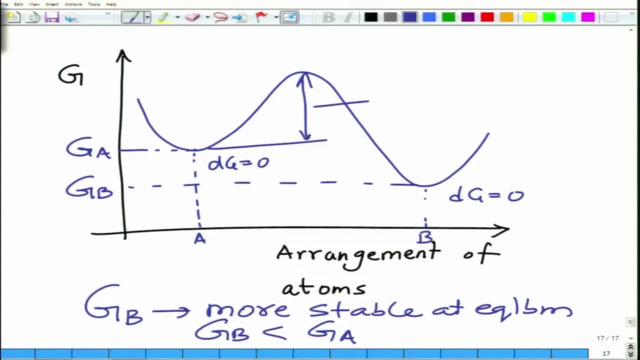 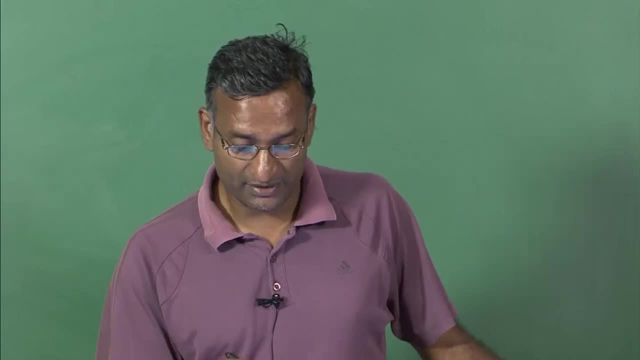 to overcome energy barrier. So this is energy barrier Delta, let us say Q. This energy has to be overcome for system to again achieve a low energy state. So as a result, typically some sort of impetus has to be provided for system. 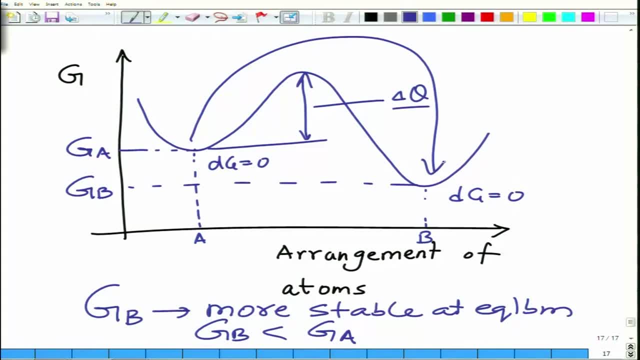 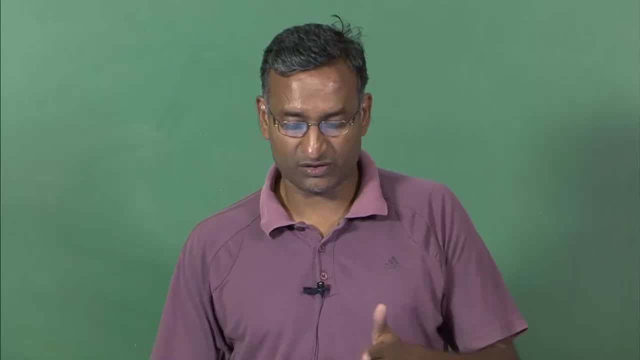 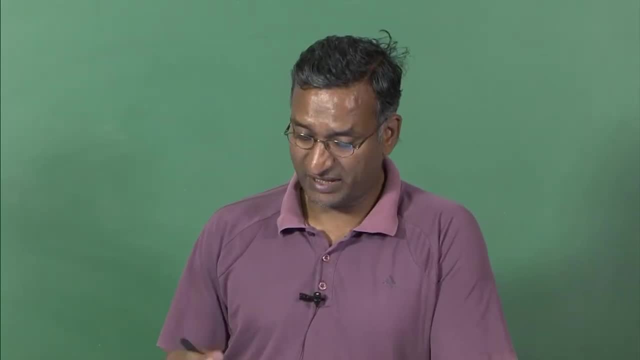 to move from this state to that state. So this happens generally in glasses. In glasses there are local minima in energy and the system stays in that energy because the delta Q can be quite large for system to achieve The proper equilibrium. However, for many crystalline systems, for many solids, the minima 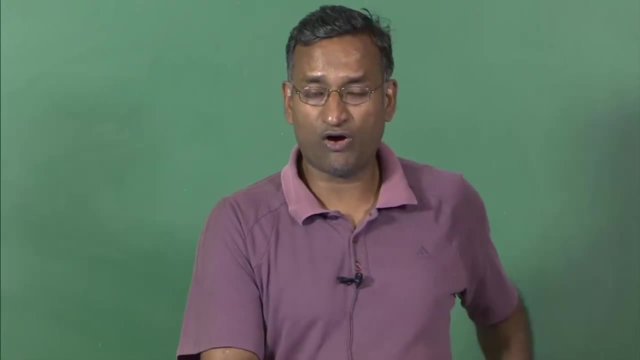 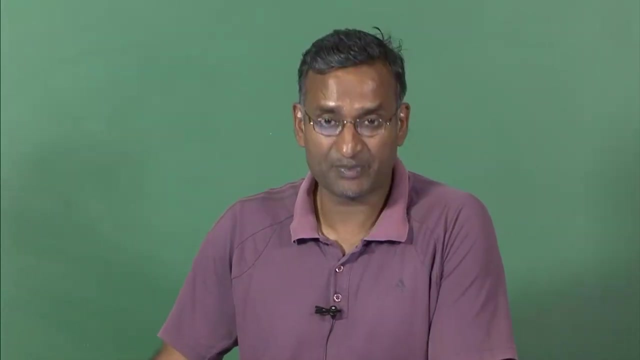 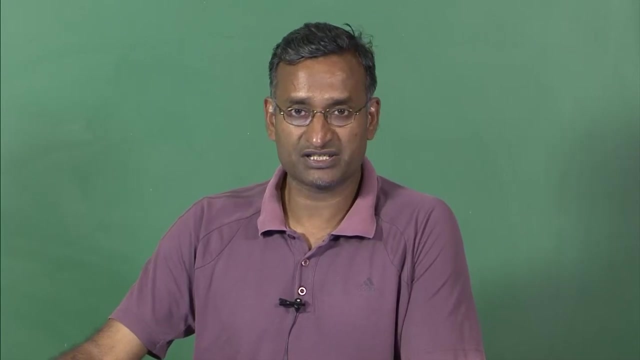 is achieved quite fast. So minima, how fast or how slow minima is achieved, that is determined by the kinetics or the time dependent rate processes within the system. But generally the tendency of a system: if you leave it enough for long, enough time, it will achieve the equilibrium. 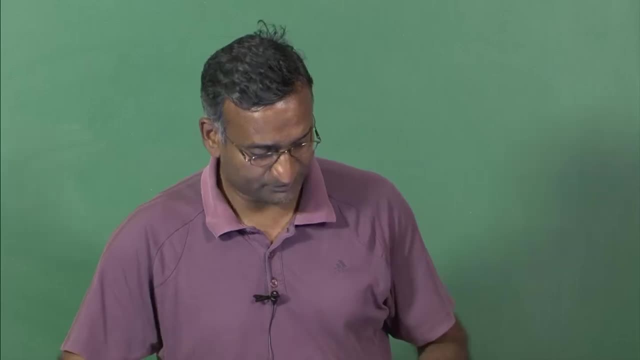 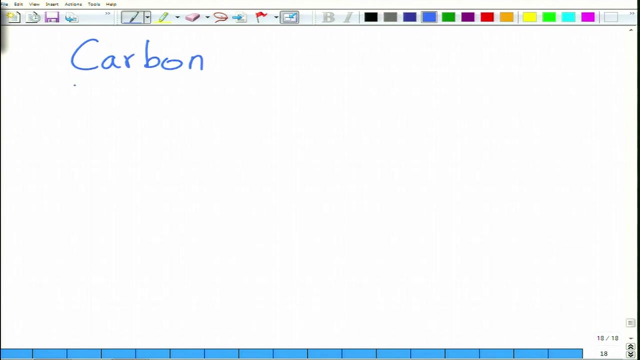 with lowest free energy state. pour example, if I give you- I will give you the example of diamond- the carbon, So carbon if you leave for a long time. the thermodynamic state, stable state of carbon is. it has two forms: One is graphite, second is diamond. 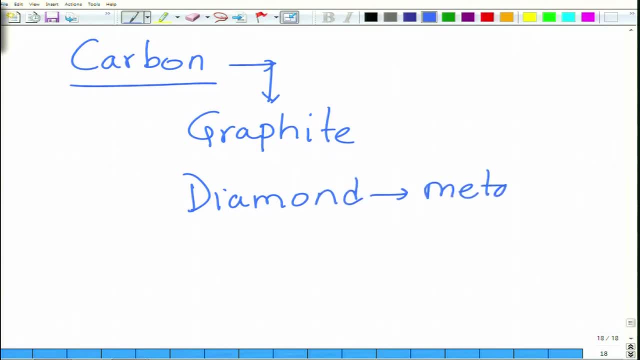 Diamond is the made as stable form and graphite is the stable form. So these are the stabilizing states, But we do see diamond exists. We do see that diamond exists and, however, if you leave diamond long time, 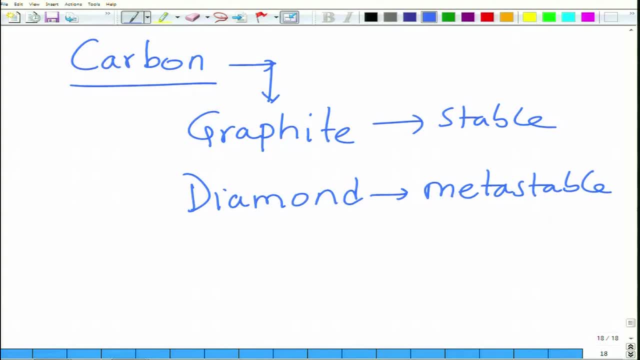 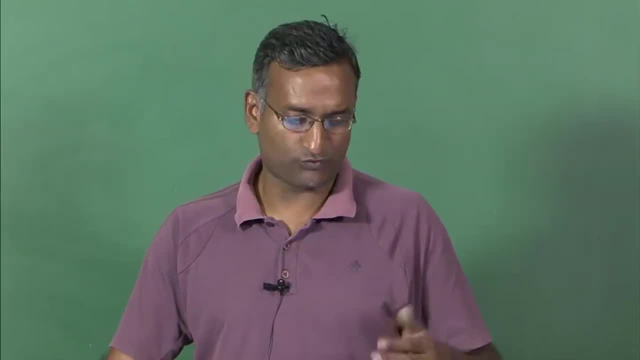 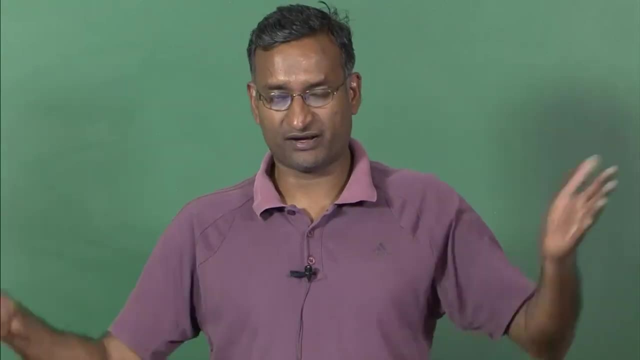 for very long time. diamond will eventually convert to graphite, But the process is so slow that virtually for very long time, virtually for eternity, the diamond appears as if it is stable, But within size of earth. the timeline of earth is very long. 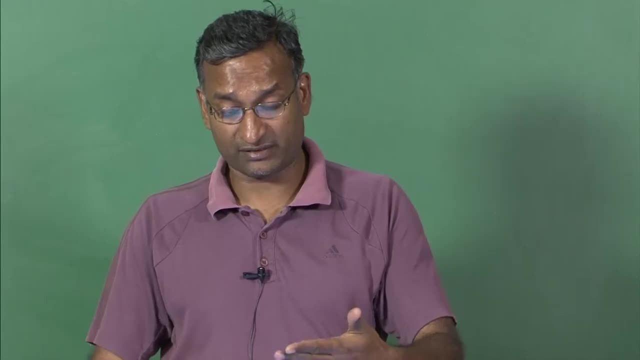 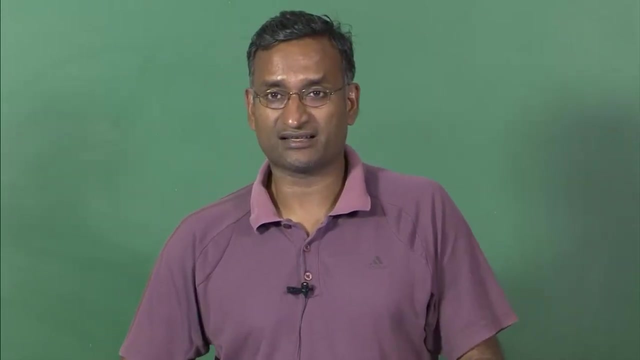 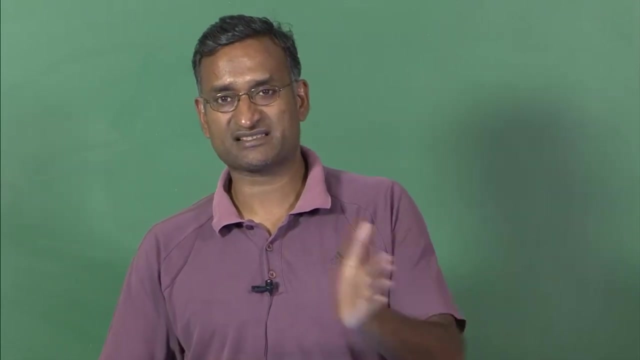 As a result, the phase transformations that happen from diamond and graphite. they don't happen in our lifetime. They take millennia for them to happen. Similarly, glasses: The crystalline glass is more stable as compared to amorphous glass, But what we see in front of us is mostly amorphous glass because the time scales at which amorphous glass 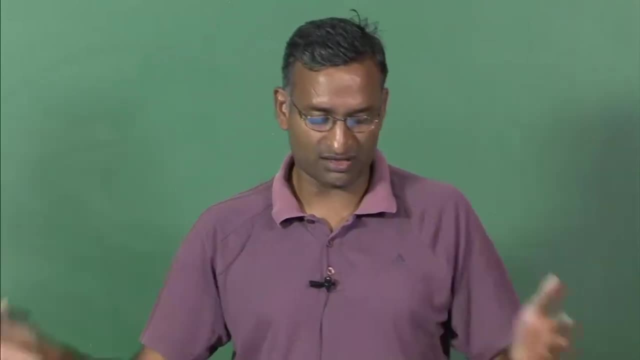 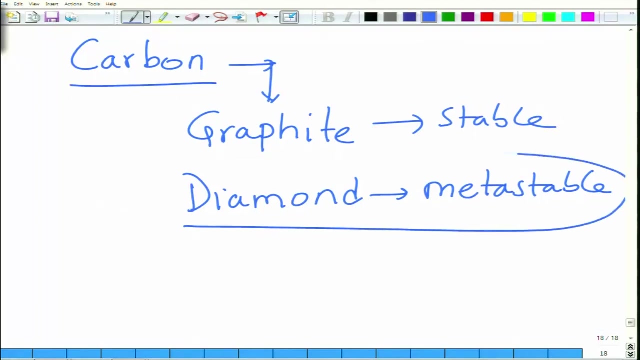 is converted into crystalline glass are huge. They are way beyond our imagination. So that is why you see these metastable states. So that is why you see these metastable states. They seem as if they appear to us, as if they are the stable phases.